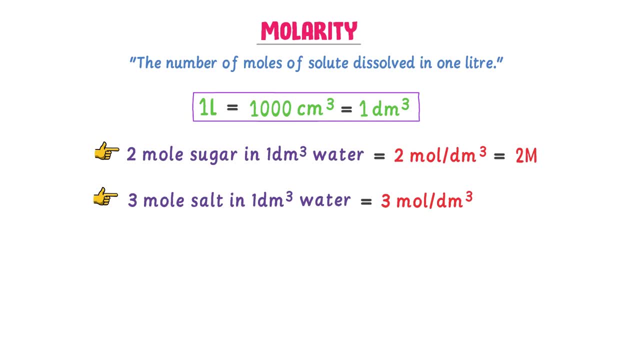 Here the concentration is 3 moles per dm3, or we just tried 3m. Thirdly, consider 10 moles of potassium hydroxide and 2 dm3 of water. Can you guess the concentration of this solution? Well, we divide the number of moles by the volume of solution. 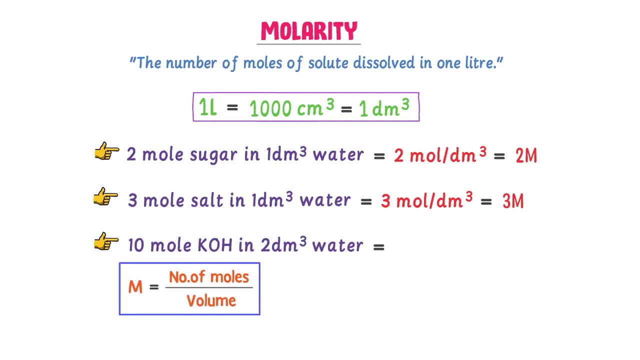 So the formula of molarity is number of moles divided by volume, or 10 moles upon 2 dm3 is equal to 5 moles per dm3, or we just tried 5m. Thus, by this way, we can easily calculate the concentration of a solution. 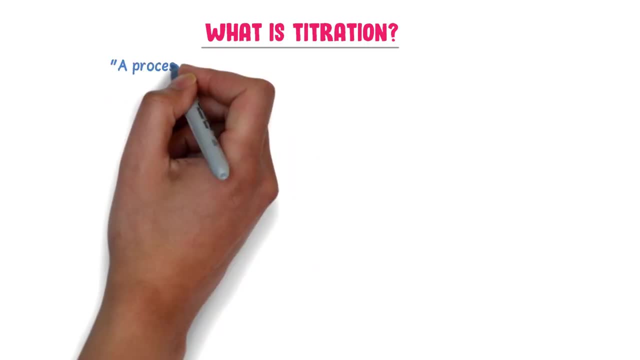 Now, what is titration in chemistry? Well, a process in which a solution of known concentration is used to determine the concentration of an atom. Well, a process in which a solution of known concentration is used to determine the concentration of an atom. 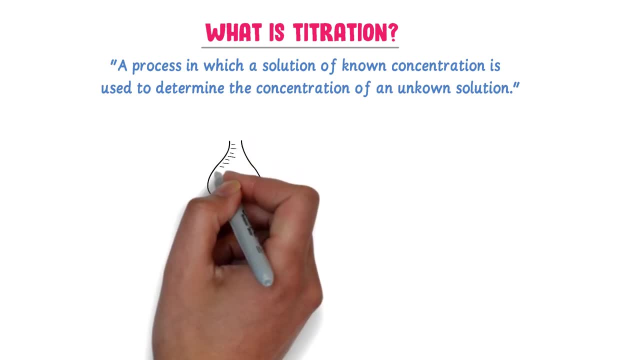 An unknown solution is called titration. For example, consider sodium hydroxide solution and HCl solution. Let the volume of sodium hydroxide taken in this object is 50 cm3 and its concentration is 0.1m, While the volume of HCl taken in this object is 30 cm3, but its concentration is unknown. 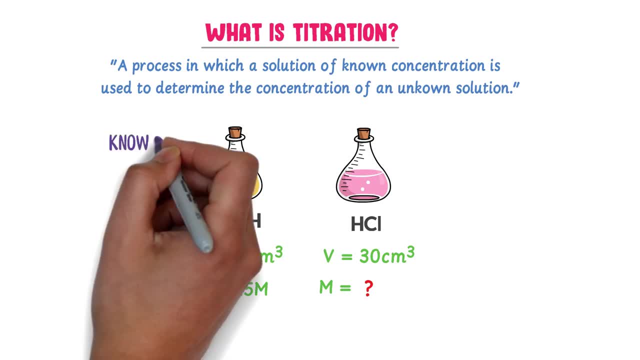 Now listen carefully. This is a solution of known concentration. It is called titrant. Let me repeat it: This is a solution of known concentration. It is called titrant, While this is a solution of unknown concentration, It is called enolate or titrant. 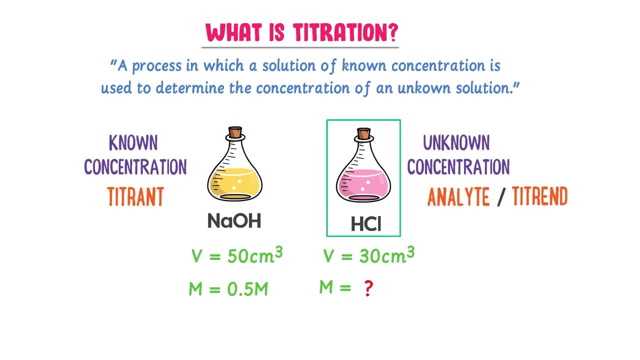 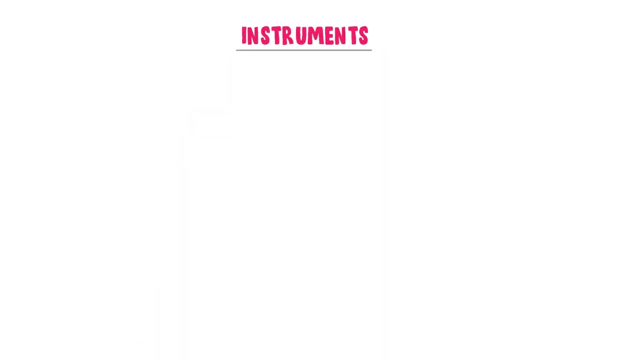 Let me repeat it: This is a solution of unknown concentration. It is called enolate or titrant. In titration We use this solution of known concentration to find the concentration of this solution. This whole process is called titration. Also, you should learn about the main instruments used in the titration. 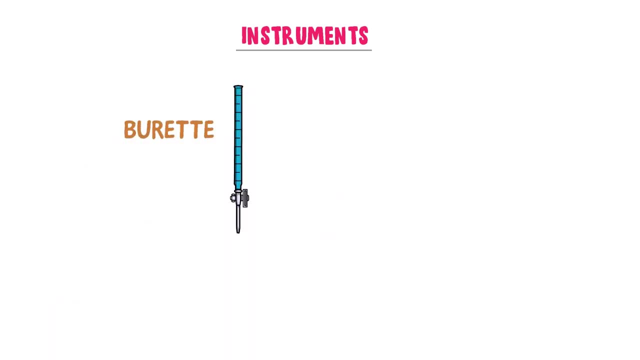 The primary instruments used in titration is burette and the other one is conical flask. In burette we take the solution of known concentration, like sodium hydroxide, Which is also known as a titrant, While in conical flask we take the solution of unknown concentration, which is also known. 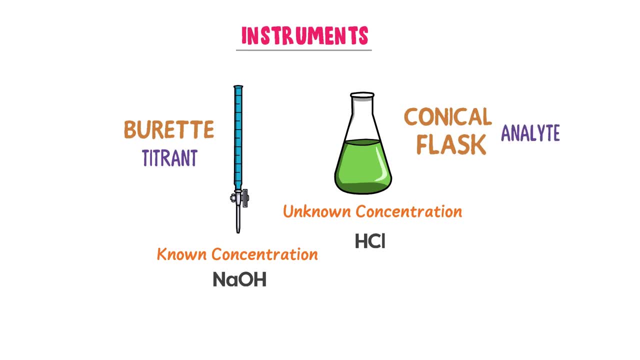 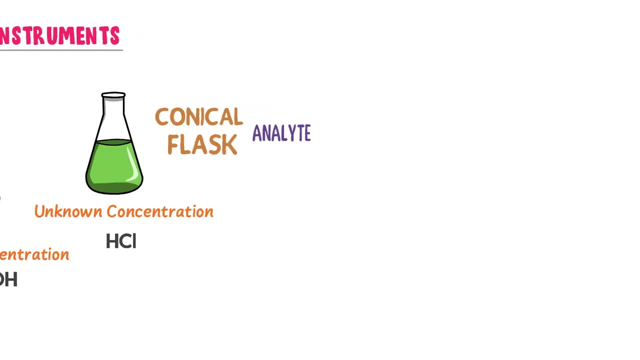 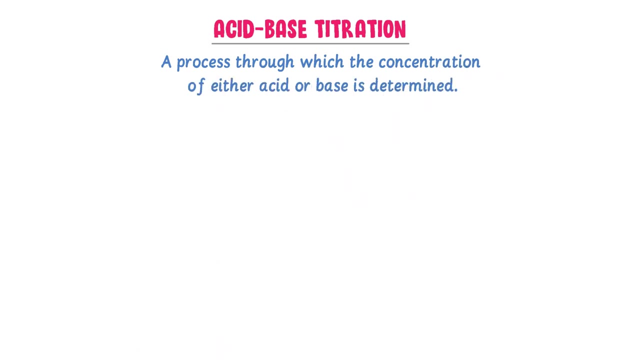 as enolate or titrant. Thus, remember that we take titrant and burette, and we take enolate and conical flask. Now, what is acid-base titration? Well, a process through which the concentration of either acid or base is determined is called titration. 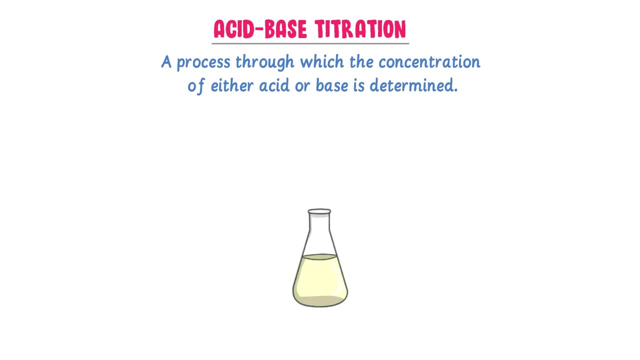 acid-base titration. For example, consider 30 cm³ of HCl solution in conical flask. If I ask you find the concentration of this 30 cm³ solution of HCl, how can you find it? Well, I take 50 cm³ of sodium hydroxide solution in burette, which has 0.5 molarity. 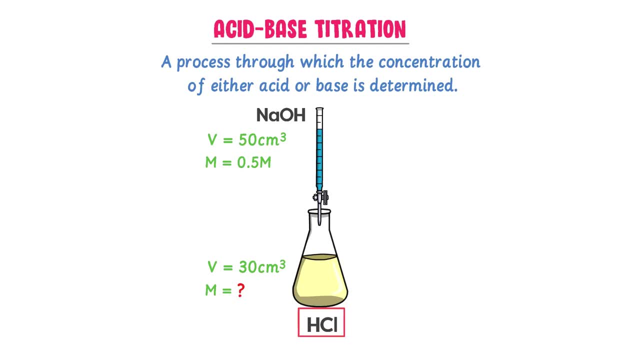 Also, we know that acid like HCl reacts with base like sodium hydroxide to form salt plus water. So we would react acid HCl with base like sodium hydroxide. Hence this whole process is called acid-base titration. We know that the volume of HCl is 30 cm³ its concentration. 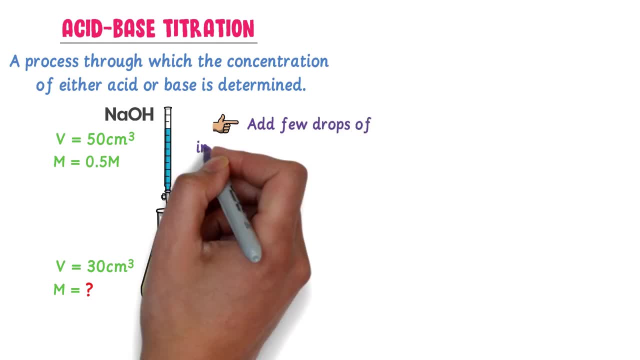 is unknown. The second step is to add few drops of intake of this solution in burette solution. I add a few drops of acid-base titration indicator to conical flask. are analyte, The indicator will show us the end point of a. 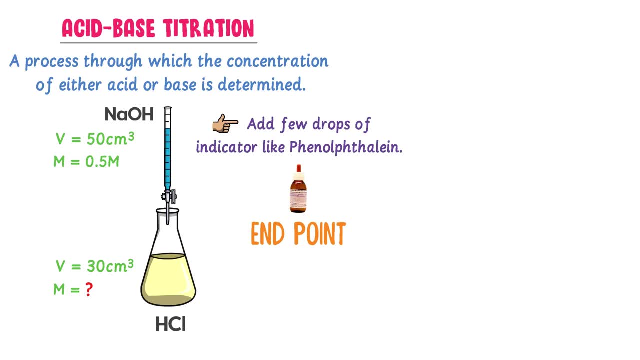 reaction between base and acid. I take indicator like phenolphthalein. The third step is to note down the initial volume of titrant sodium hydroxide and the burette. We can see that the initial volume of titrant sodium hydroxide is 50 cm3.. 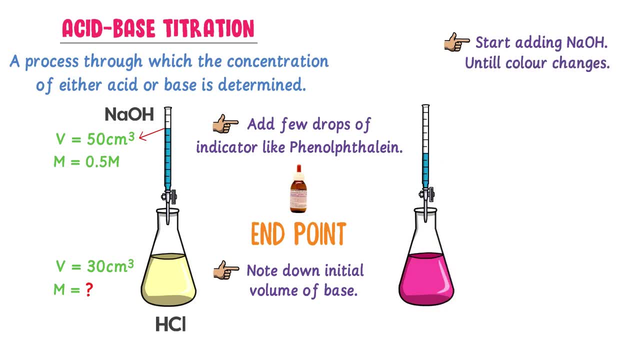 The fourth step is to start adding the titrant sodium hydroxide to the analyte HCl until the color changes. For example, when we add sodium hydroxide to the HCl, they will react together and the color of indicator would change from colorless to deep pink. This color change 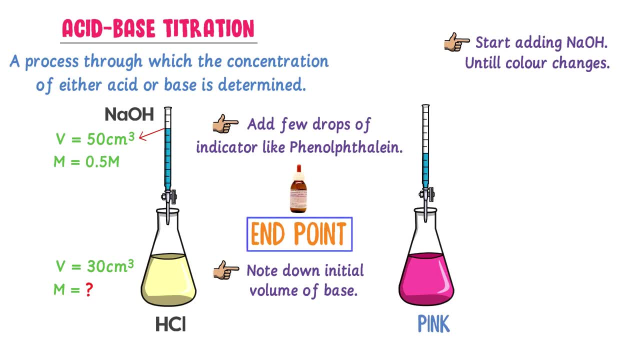 indicates the end point or completion of acid-base reaction and we would stop further addition of titrant. The fifth step is to note down the final volume of titrant. For example, the final volume of titrant is 30 cm3.. The last and the sixth step is to find the volume of titrant sodium hydroxide used to 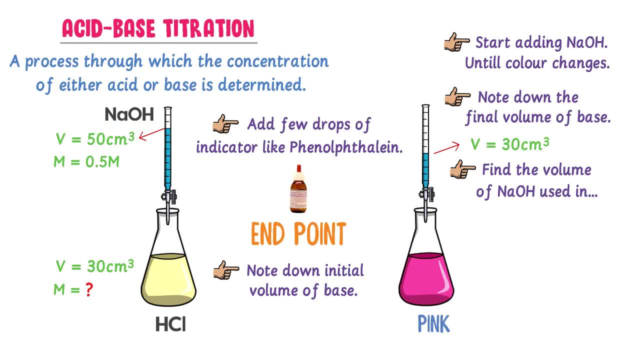 react. with analyte HCl, For example, the initial volume of titrant was 50 cm3 and the final volume of titrant was 50 cm3.. The final volume of titrant is 30 cm3.. So always subtract final volume from the initial. 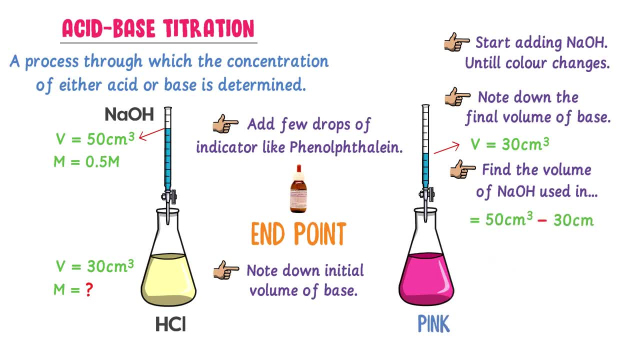 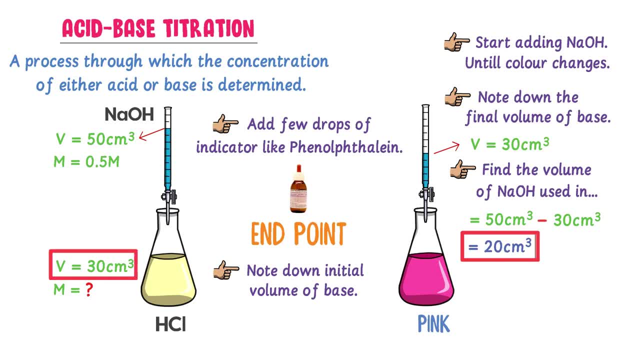 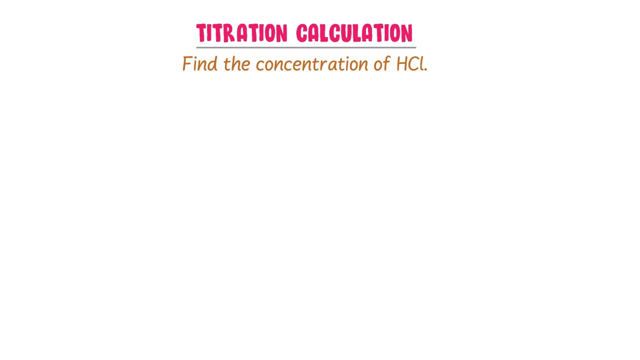 got 30 cm3 solution of sodium hydroxide, react with 30 cm3 solution of HCl to neutralize it completely. Thus noted down this important point. Now the final step is titration, calculation, or find the concentration of HCl. Firstly, 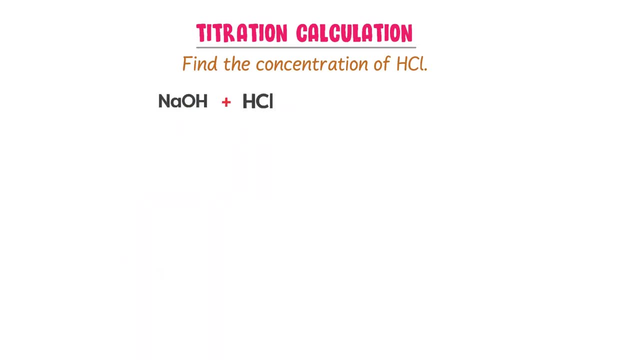 I write the chemical reaction. Sodium hydroxide plus HCl react together to form sodium chloride plus water. Secondly, I balance this chemical reaction. If you do not know balancing chemical reaction, watch our video and its link is given in the description. 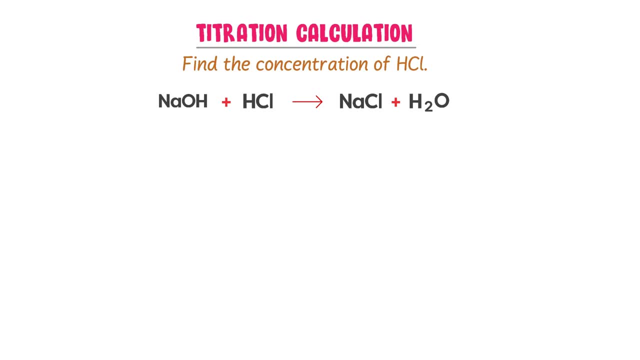 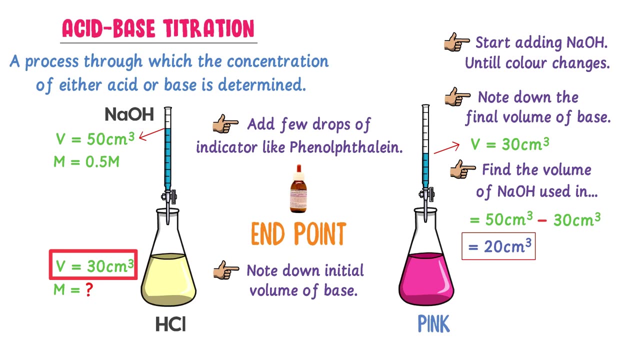 We can see that this chemical reaction is already balanced In the previous slide. we know that 30 cm cube solution of HCl is used and 20 cm cube of sodium hydroxide solution completely react with it having 0.5 molarity. 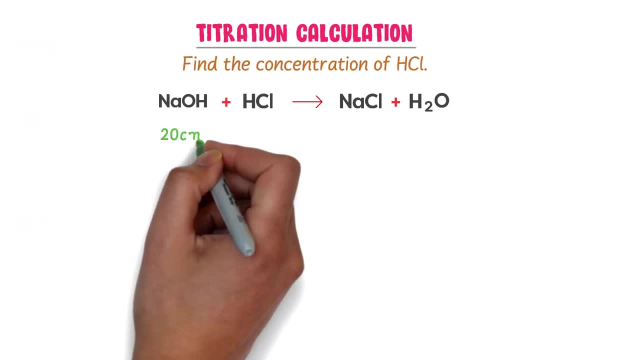 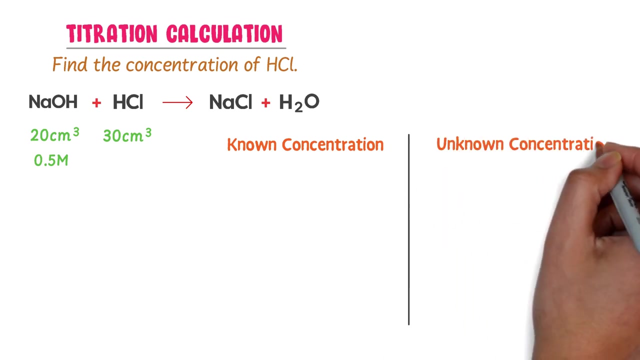 So I write here: volume of sodium hydroxide is 20 cm cube, volume of HCl is 30 cm cube and the concentration of sodium hydroxide is 0.5 m. Here I write non-concentration and here I write unknown concentration. 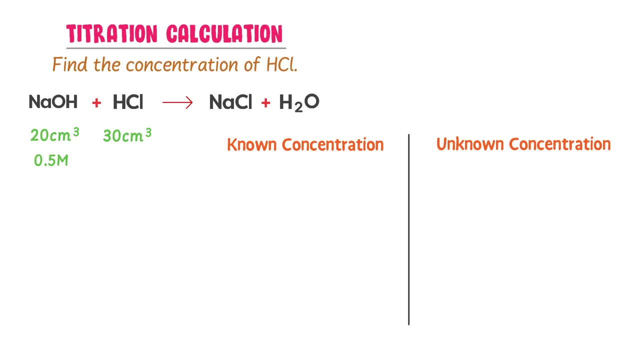 The non-concentration is sodium hydroxide And the unknown concentration is HCl. Firstly, I convert the volume of sodium hydroxide to dm cube. I write 20 cm cube divided by 1000.. I get 0.02 dm cube. 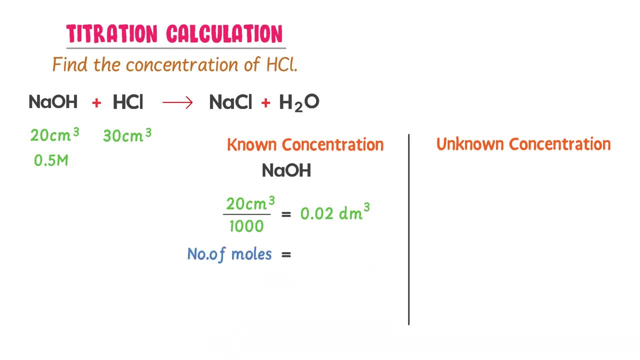 Then I find the number of moles of sodium hydroxide used, which is equal to concentration into volume. The concentration of sodium hydroxide is 0.5 m And its volume is 0.5 m. The volume is 0.02 dm cube. 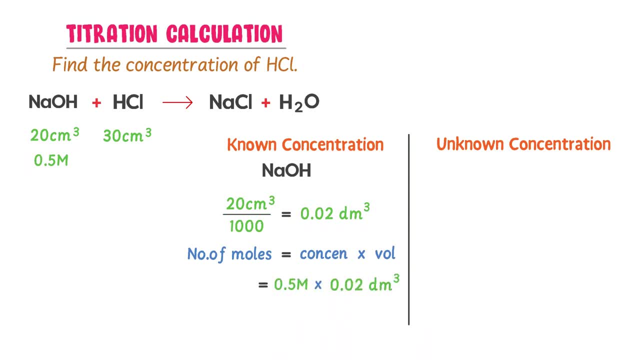 I write 0.5 into 0.02.. So I get 0.01 mol. The 0.01 mol of sodium hydroxide has reacted with HCl. On the other hand, I also convert the volume of HCl into dm cube. 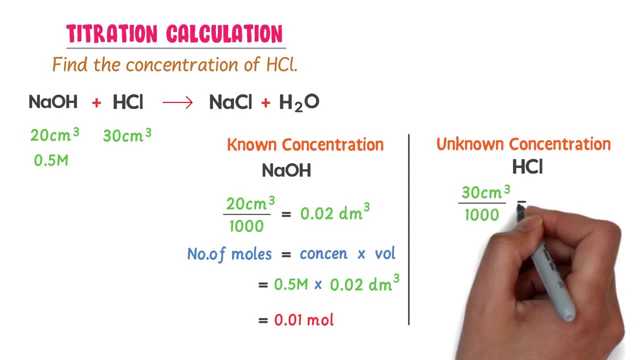 30 cm cube divided by 1000. I get 0.03 dm cube. Now listen carefully. 1 mol of sodium hydroxide react with 1 mol of HCl. So the ratio of number of moles between them is 1 to 1.. 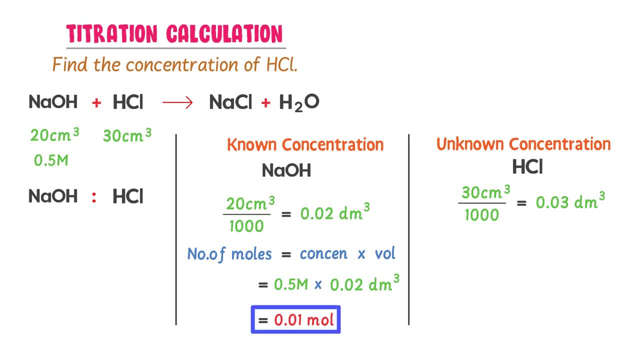 We know that 0.01 mol of sodium hydroxide has reacted. I write here 0.01 mol. The ratio is 1 to 1.. I also write here 0.01.. So the number of moles of HCl reacted with sodium hydroxide is 0.01 mol. 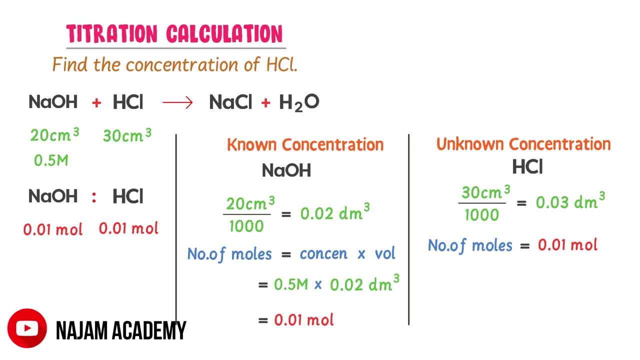 The ratio is 1 to 1.. I also write here 0.01.. Now we can easily calculate the concentration of HCl. We know that concentration is equal to number of moles upon volume. The number of moles is 0.01 and the volume of HCl is 0.03 dm cube. 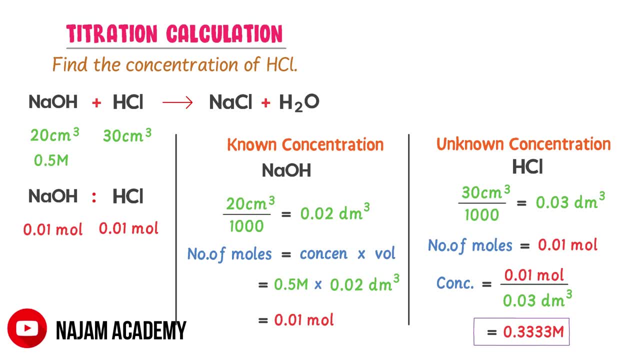 So we get 0.33 moles per dm cube, or 0.33 m. Thus this is the concentration of HCl. I hope that you liked this video. I hope that you have learnt all about the titration.